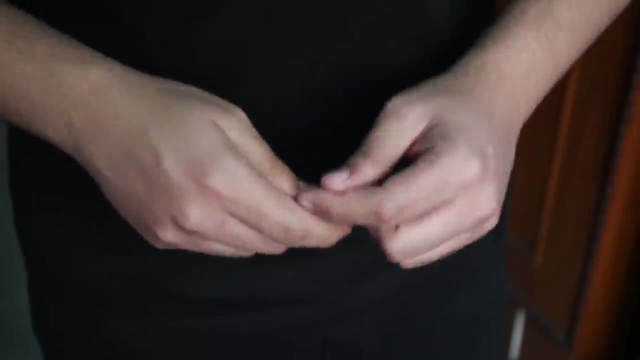 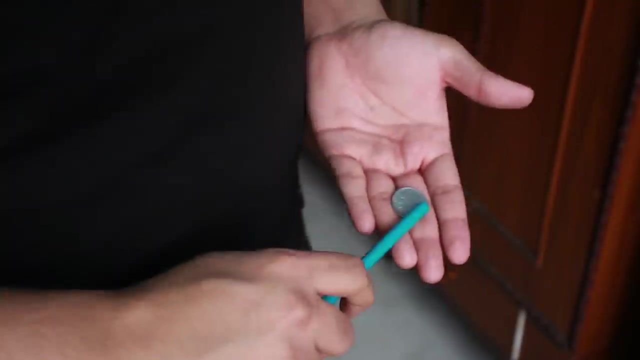 Other hand. so that's how you're going to do the first trick. Now, moving on to the second one, it looks somewhat like this: You have a coin over here and you have a pen. now watch one, two, three. The coin has vanished, just like that. now, in order to bring the coin back, all you have to do is just 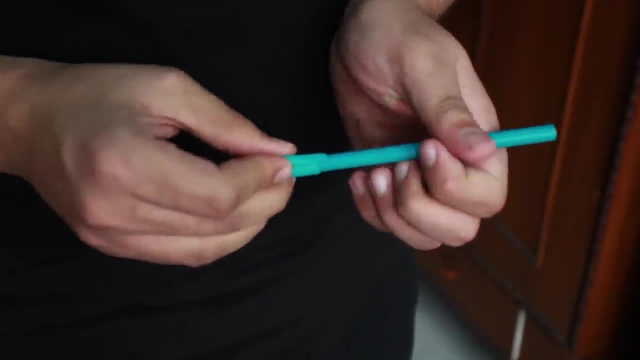 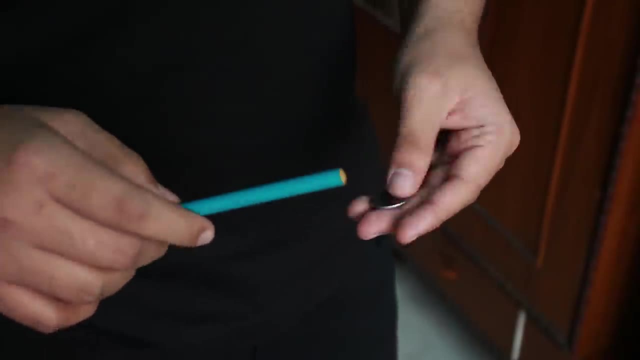 Shake the cap and the coin falls from inside of it. So that is the second trick that always fools anyone. This trick is another easy trick, and here is how you're going to do it: You have to keep a coin on one of your hands and you have to hold. 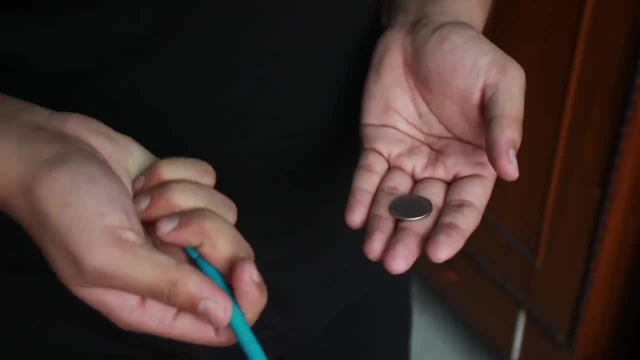 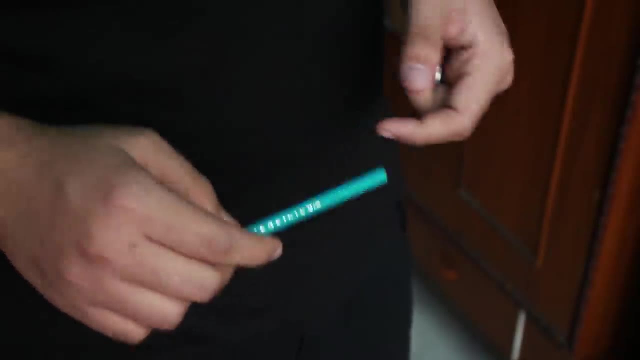 The pen with the other hand and the cap side will be inside your hand. So, basically, that's going to be the starting point, and then what you're doing is basically You're going to turn like this, with the pen side towards the spectator, because that is the best angle, and then what you're going to do 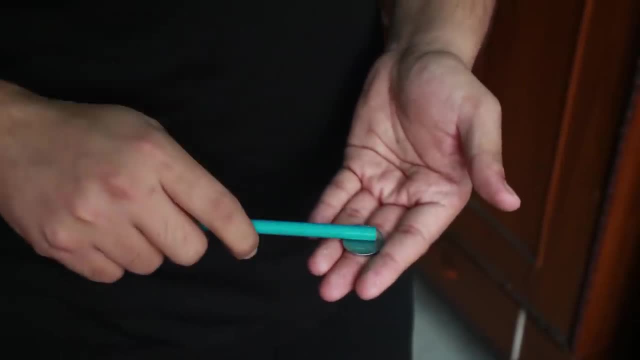 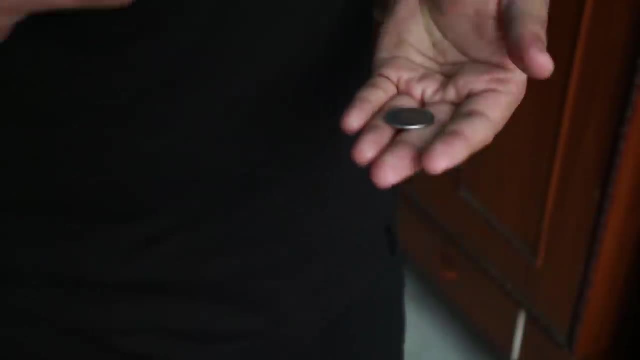 Is you're going to tap on the coin three times. so the first two times you actually tap on it And you also move both of your hands like that. on the third time, All you do is basically throw the coin up and you go down fast. So in that movement you actually catch the coin inside the other hand. 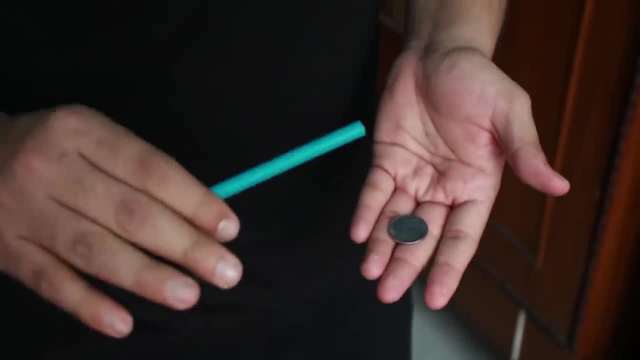 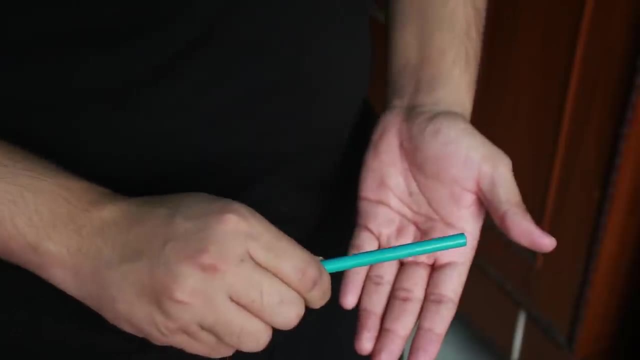 So I'll just try to give you a slow-motion view, but this is not going to look good because this camera is not a slow-motion camera. So, anyways, this is what it looks like. I'll try to do it in the slow motion, So I don't know if that was perfect or not, but basically that's it. 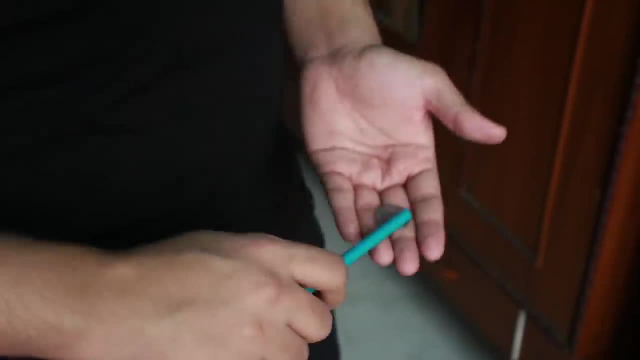 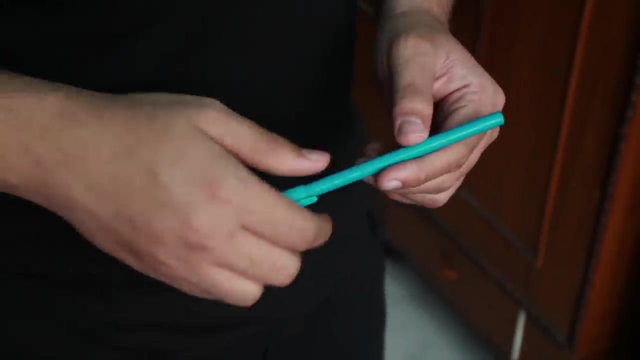 That's what happens, and that happens in this angle and in a fast motion, So it looks like that the coin has vanished and the coin is actually basically in this hand. now all you do is basically, from this hand, you hold the pen like that and Keeping the coin in the palms position. 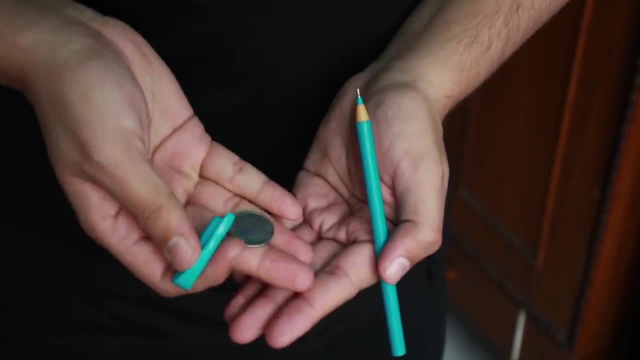 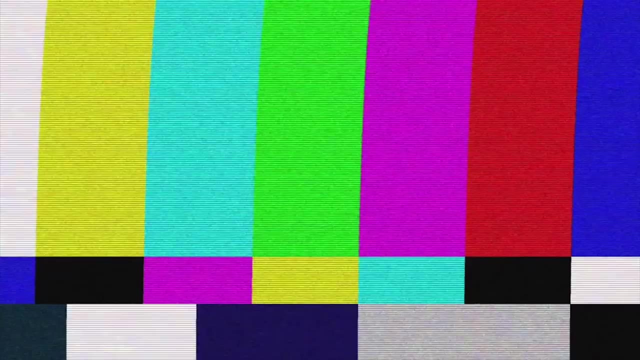 You open up the cap and then, while you shake the cap, All you do is basically open these fingers and the coin drops onto this hand. So basically, like that, you are going to do this trick. The next one is the pen and the ring trick. So I'm going to take the pen and I'm going to keep it over here. 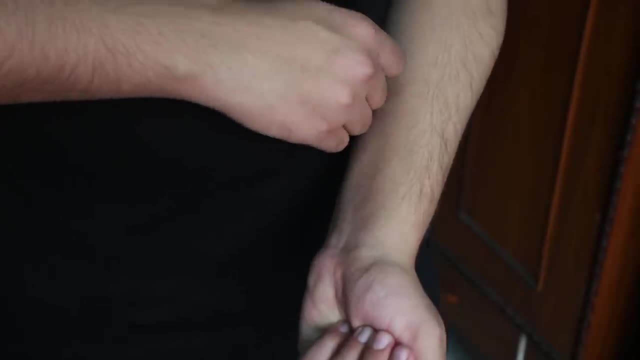 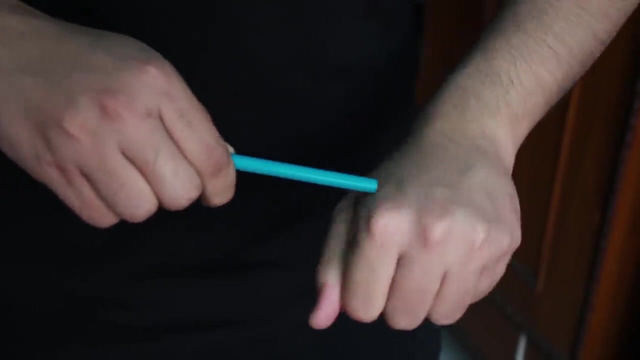 Then I'm going to take this ring and I'm just going to take it in this hand. Then I'm going to take this pen and all I'm going to do is basically move this pen Just like a magic wand over this hand, and all that does is it actually makes this ring disappear. 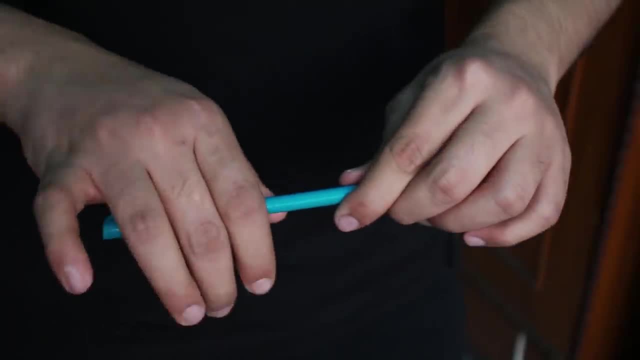 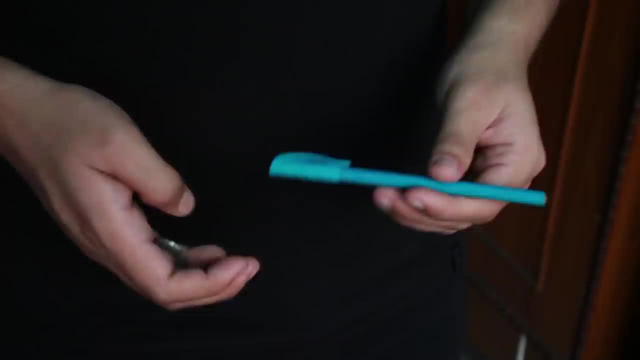 So that makes the ring disappear, but the ring actually Comes To this position. So that is the pen and the ring trick, and here is how you'r going to do it. Now, in order to do this trick, all you need is a pen and a ring. Now, both of these things could be borrowed. 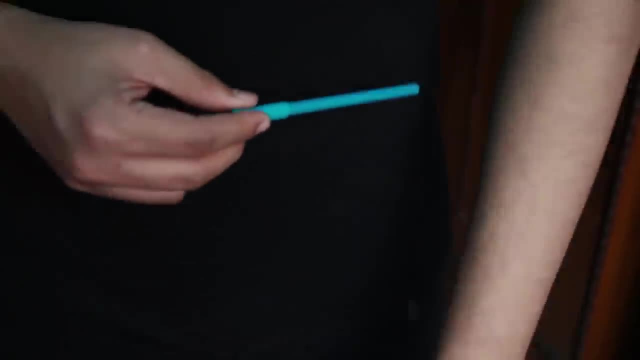 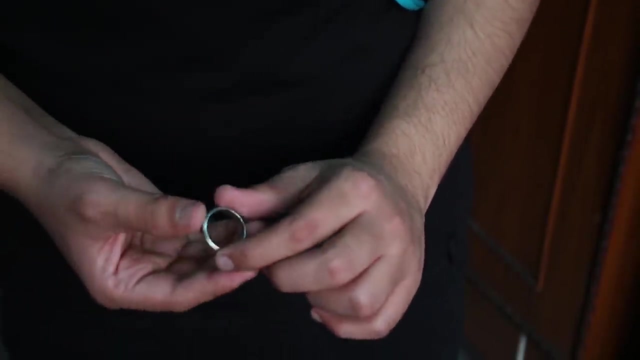 So it really doesn't matter. After you take that, take the pen and hold it by the side of your body With the help of your arm- and that is very important- and then, after that, all you're going to do is basically a retention technique with the ring. 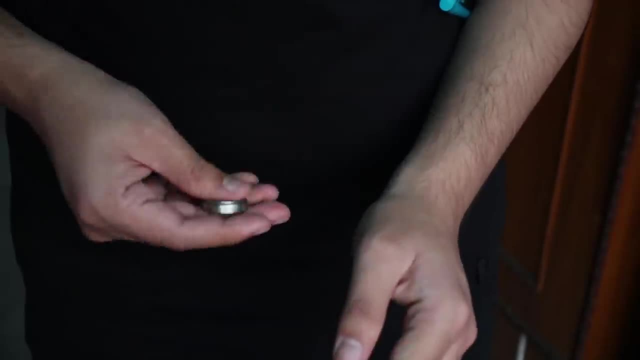 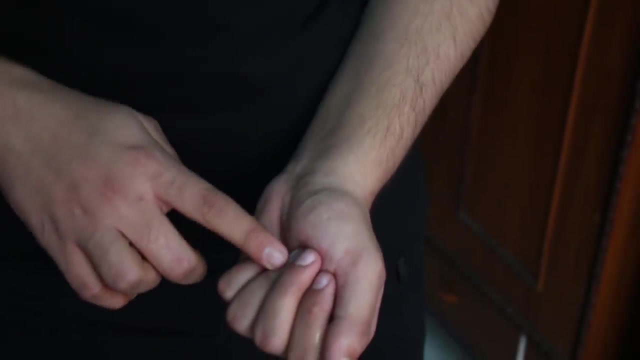 In your other hand. So basically, the French drop, or you can do the thumb palming which I did in the performance. you can do it. so the spectators will think that the ring is over here now. as the spectators think that the ring is over here, you can actually do a. 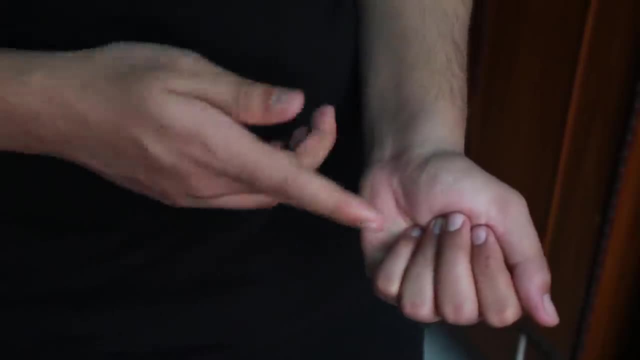 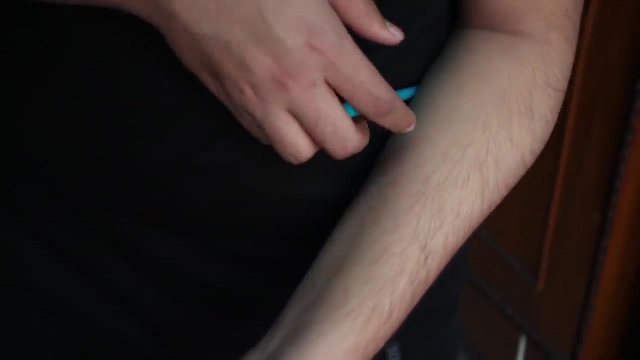 misdirection and just tap on this hand so they are going to look over here and you can actually adjust the ring over here in this hand, which is still over here, and then all you're doing is basically, when you're going to bring the pen- that is why I said that keep the pen by the side of your body when you're- 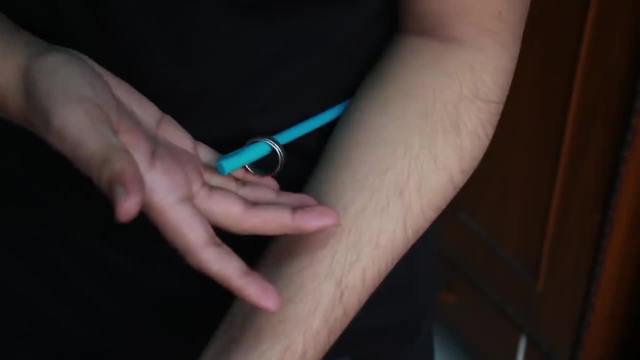 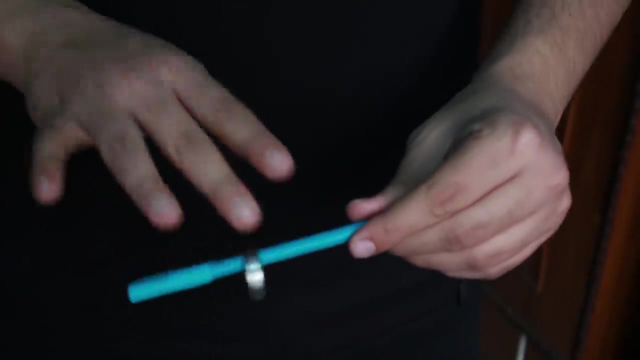 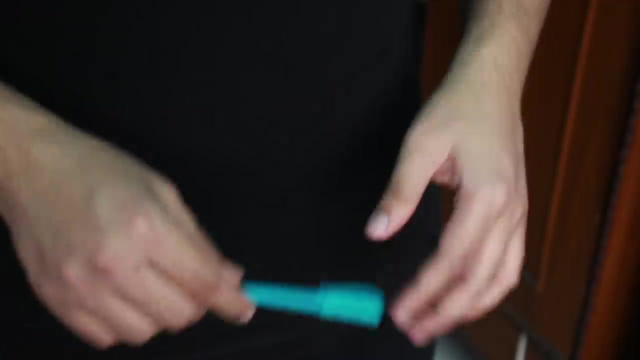 going to bring this pen. you're actually putting the ring onto the pen, just like that, and then you're holding the pen and bringing it out and then the rest of the thing as performance, just do it as the performance. so that is how you are going to do this pen and ring trick. moving on to the next one, you can see I have this. 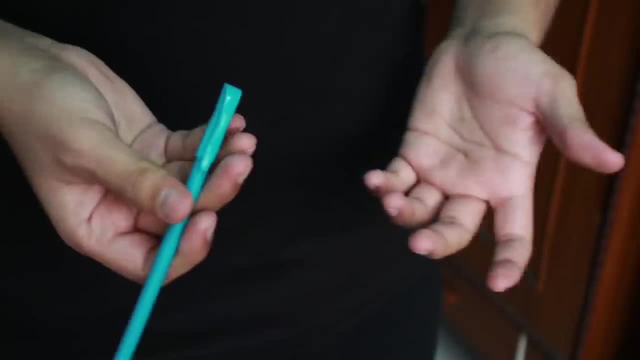 pen with a cap, just like that, and all I'm gonna do is, basically, I'm going to take this pen and I'm actually going to open up the cap, just like that, and then I'm going to wave this pen, and then I'm going to take this pen and then I'm 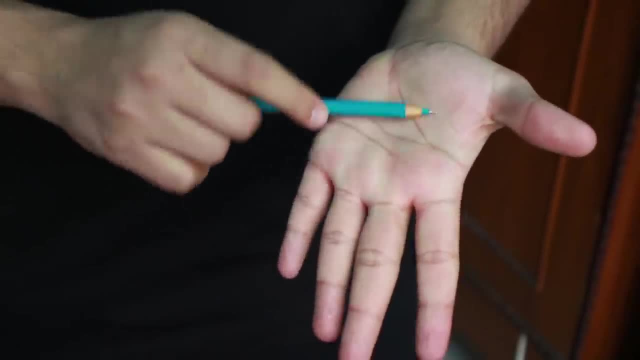 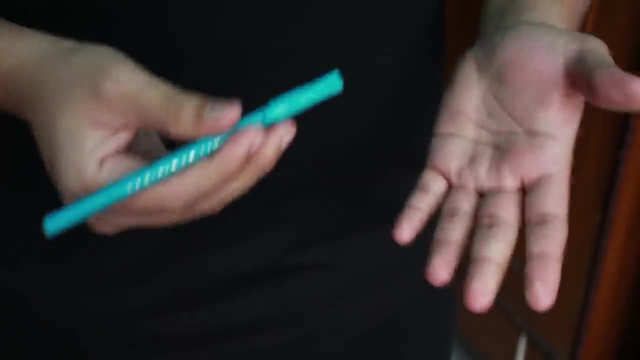 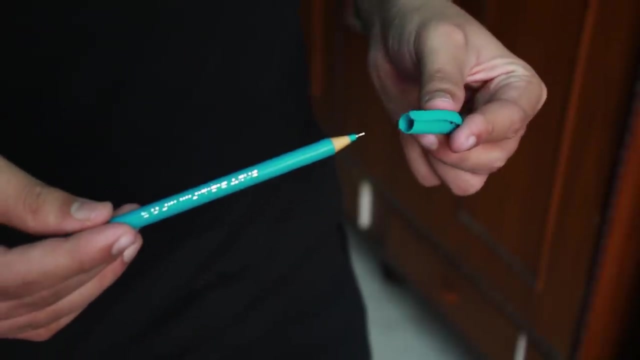 going to pull it to the side and if I get this cap it's actually gonna come up right. you can actually see that this pen is getting higher because this pen is actually gonna reach right above that hand and the cap is actually going to disappear magically from that hand and land on the back of the pen. so that is. 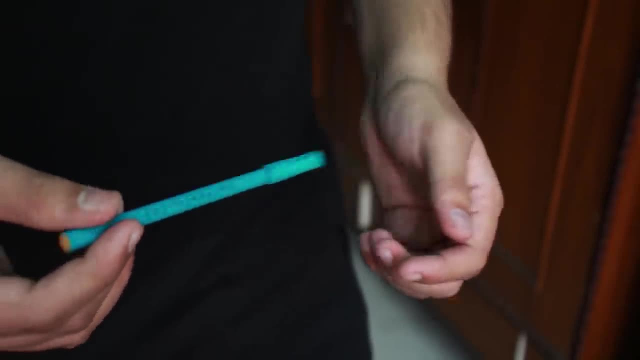 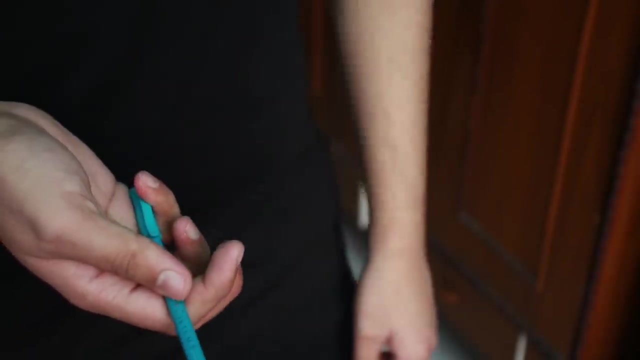 the trick, and here is how you're gonna do it. this is actually the most simple trick. all you need to do is you need to have a pen with a cap, and then what you're going to do is basically, you're going to put the cap very lightly over. 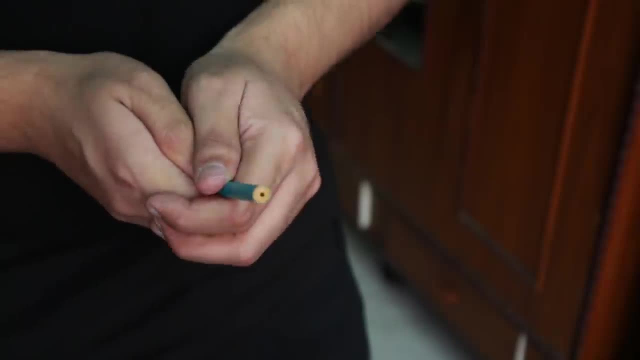 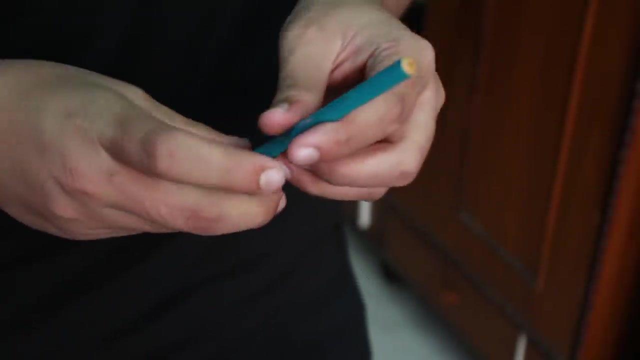 now, while you're moving this pen from this hand to this hand, you're doing it in this way, and while you're doing it, you're actually pulling the cap back with this hand, so the cap stays with this hand. it's kind of like a retention technique, so that happens. when the other hand comes, it goes. 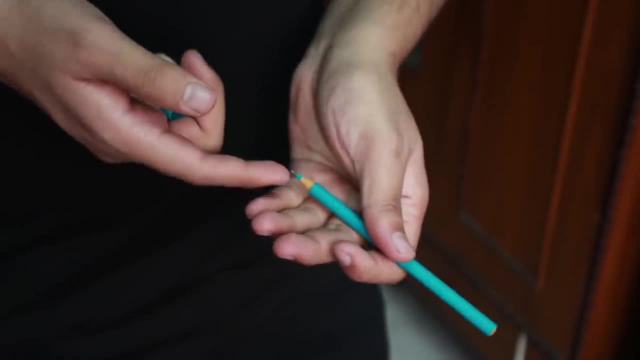 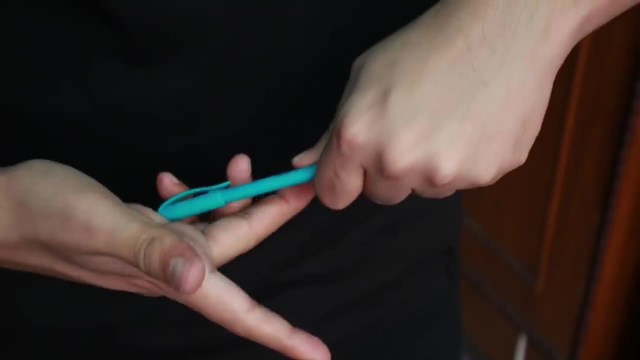 to take the pen and it takes the pen, not the cap. so the nip is over here and the pen is in this hand, just like that. and when i'm holding the pen with the other hand, i'm actually putting the cap onto the back of the pen and i'm holding it. so i'm just pretending to open the cap and then i'm 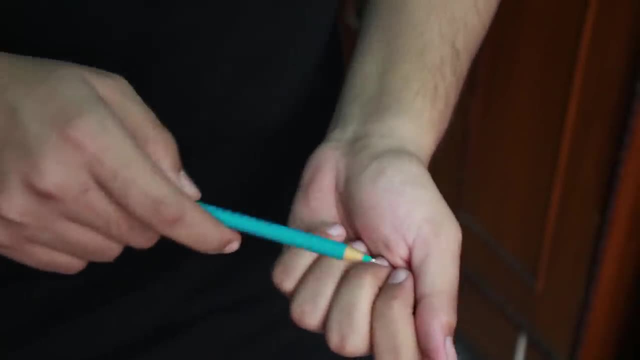 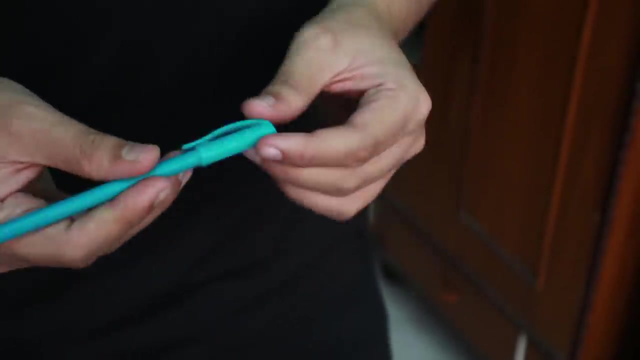 going to wave this pen and the cap is not actually present over here. so you can do it, do a magical reveal, and then you can just show the back of the pen and say that the cap has magically traveled to the back of the pen and this time, while you open it, try to make it look like that the cap was. 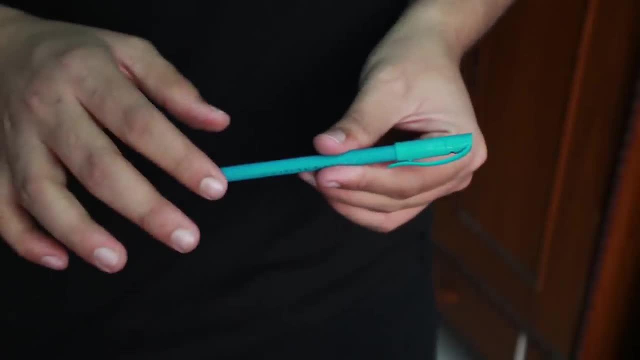 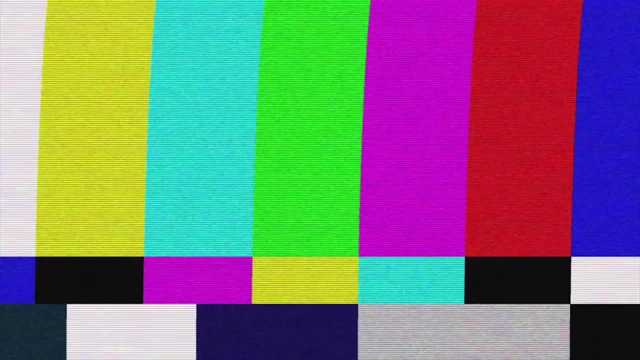 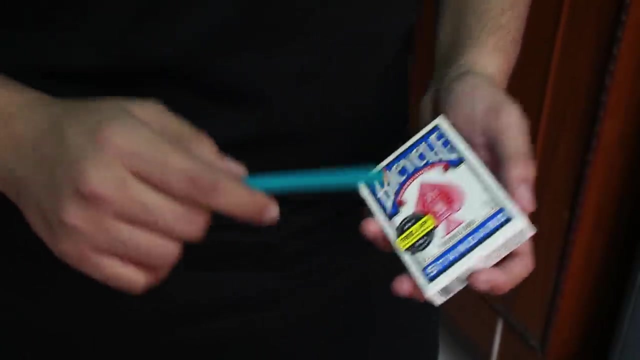 very much hardly attached to the back of it so that the spectators believe that the cap has magically went over there and you did not put it right over there. so that is the fourth one. this is the most oldest trick and it actually works when you perform this in real life, right in front of the spectators eyes. so i don't really 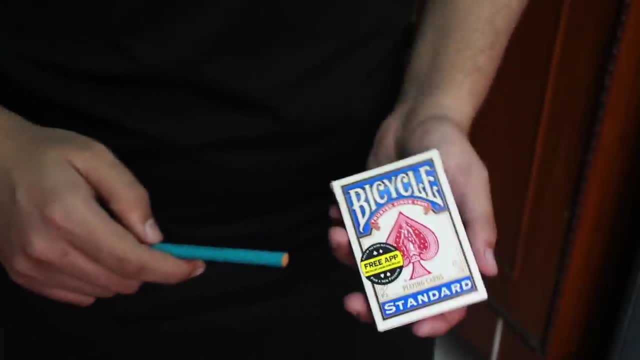 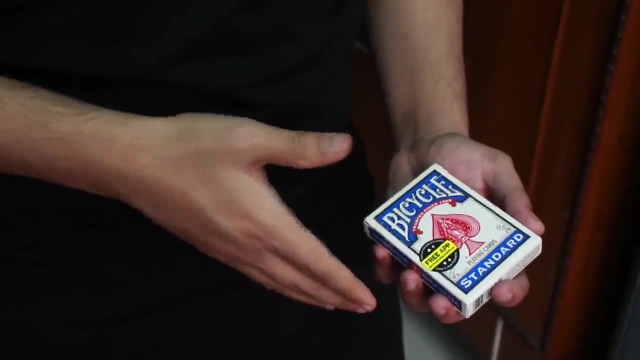 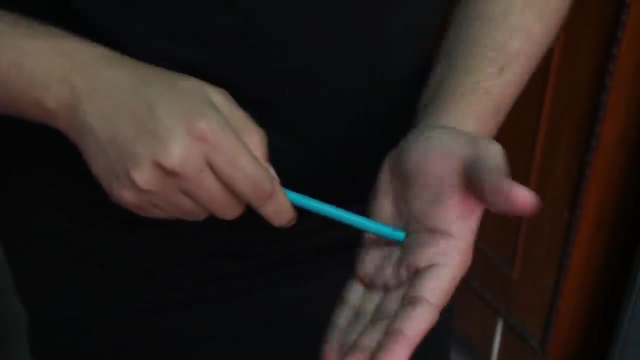 know how it will look on camera, but i'll try my best. so i have this deck of cards and i'm going to try to vanish it with the help of this pen. now watch one, two, three. i actually hit the pen behind my ears, as you can see, but watch. if i strike the pen on the deck of cards, it actually 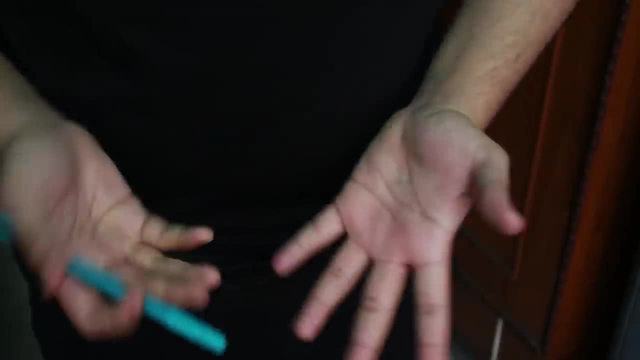 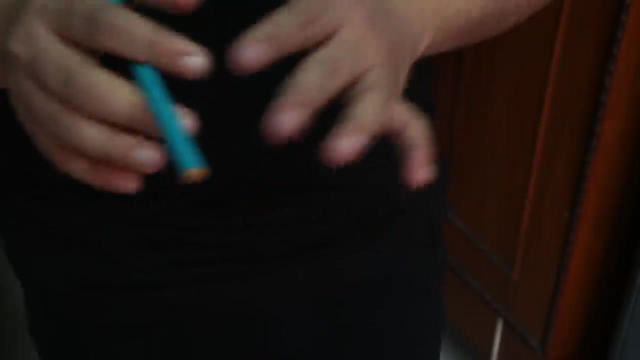 vanishes, and you can see right now my hands are empty. i don't have the deck of cards with me anymore. so that's one of the most lamest tricks on camera, but trust me, when you're going to perform this in front of the spectator, you're going to get amazing reactions. the concept behind this trick: 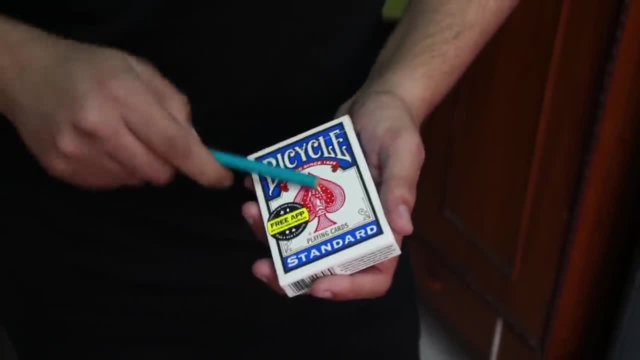 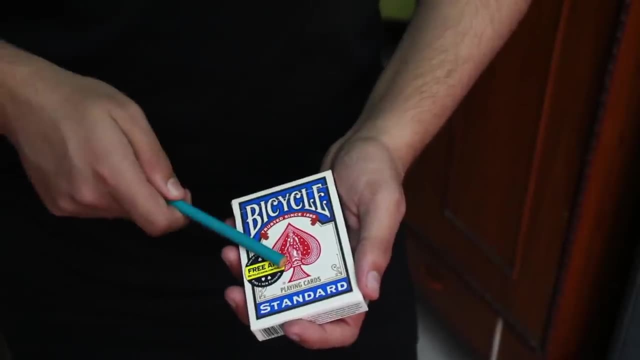 is very easy. all you have to do is you have to have a pen and any other object. you can also use any small object except for the deck of cards. so you're going to hold that object and then you're going to strike the pen three times. so the first time you strike, the second time you strike, and